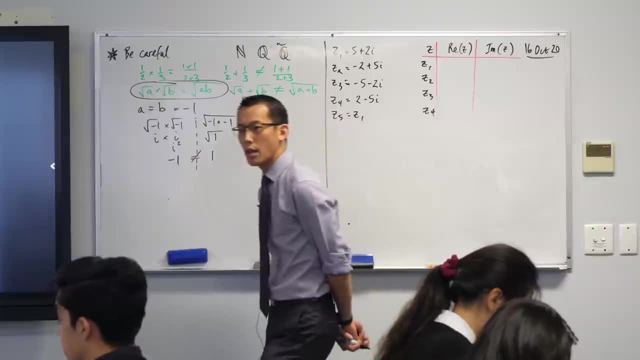 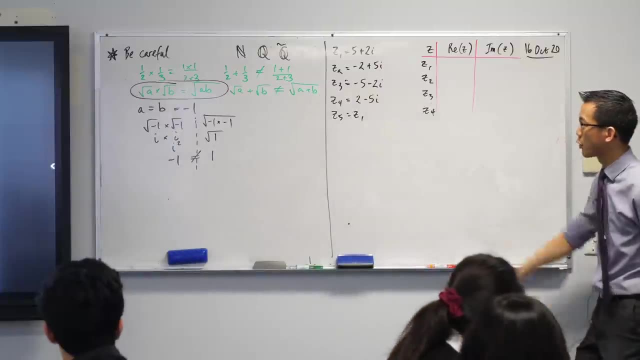 Z5 off of this list because it's clearly the same as the top row For each of these numbers. what's the real part? What's the imaginary part? Start me off. Z1.. Real component is 5.. Imaginary component is 2.. Next one, Z2.. 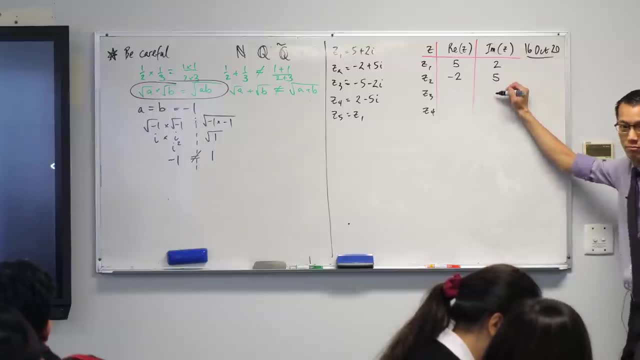 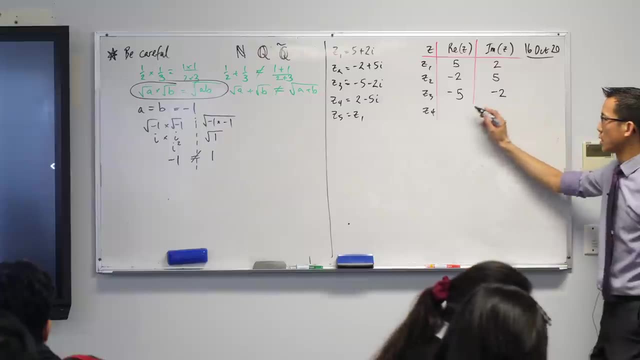 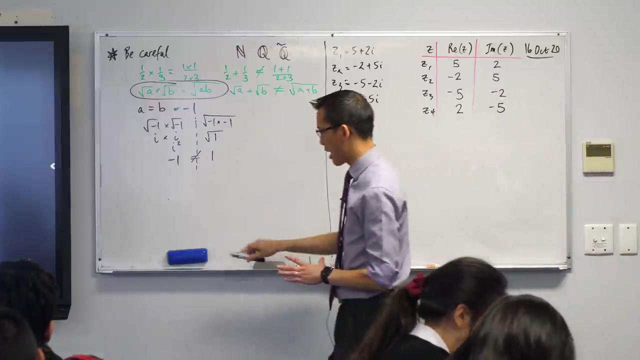 Negative 2 and positive 5.. Yeah, Next one down: Negative 5, negative 2.. Last one here: 2 and negative 5.. You okay with that? I want you to stare really hard. I'm inviting you to kind of be like. 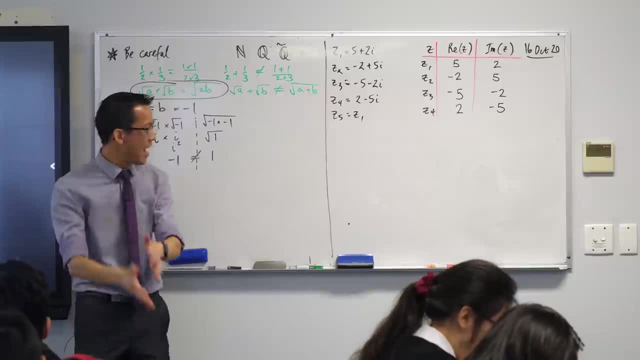 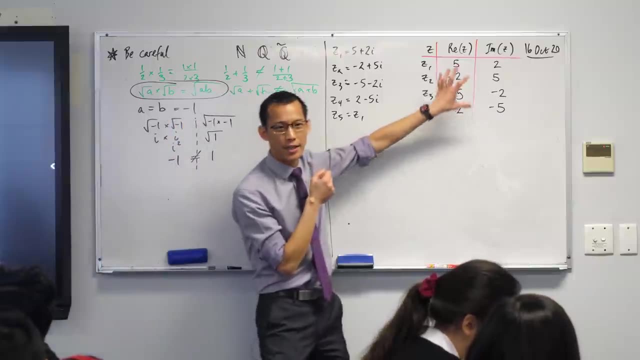 Brown, like that botanist who was staring down his microscope and he was like: What's going on here? Is there something more than what I can see? Is there something invisible underneath this that's driving this process? These are not just random numbers, right? What do you notice? What do you wonder when you have a look at these? 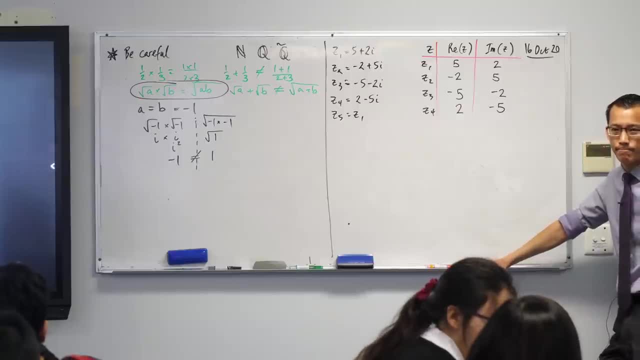 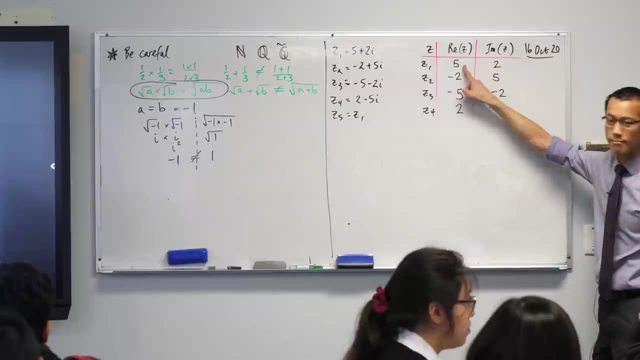 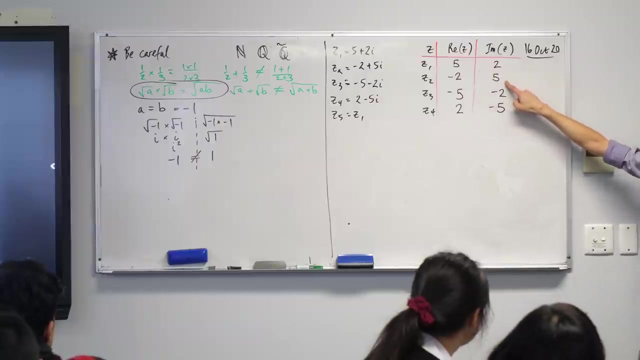 Does anyone notice any patterns? What do you see? What do you think? Start us off? Huh, okay, so real part of this, one imaginary part of this one Real part, imaginary part, real part, imaginary part, and you could extend it all the way around, right? 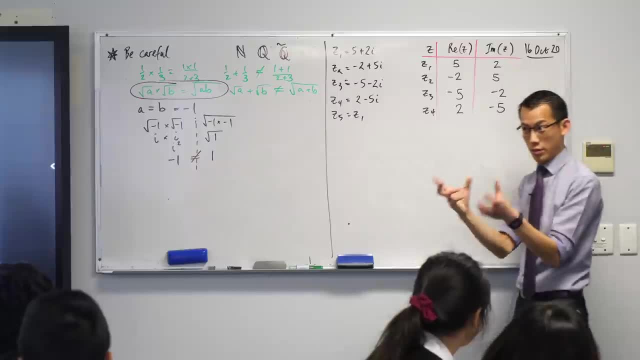 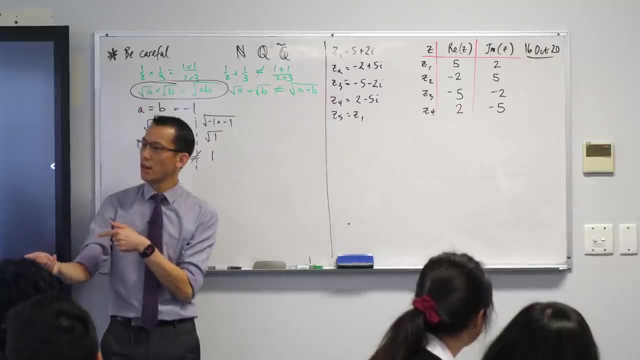 Here comes the real part and then the imaginary part. Good, So we're noticing, there's this relationship. Is there anything else that you notice? Every two cycles it multiplies by minus 4.. Every two cycles, Let me say that again, Angad, Every two cycles of multiplying by i. 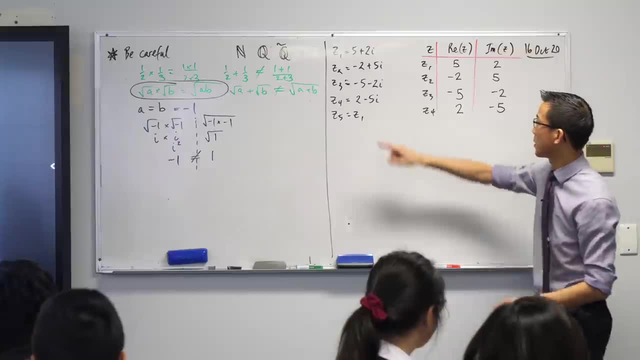 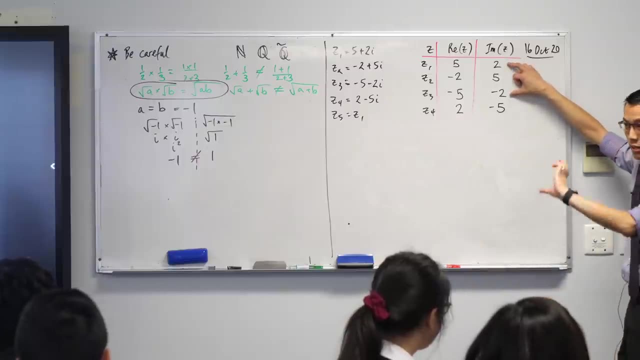 you're essentially multiplying by minus 1.. That makes sense because each time we progress, we're multiplying by i. So if you do it twice, you're multiplying by i squared. So if you have a look at these two, yeah, you see the flipping of signs. If you look at these two, 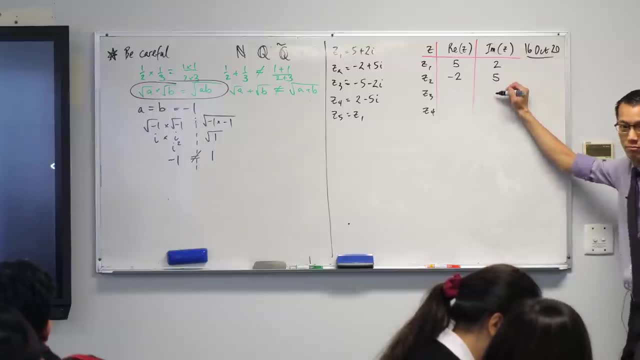 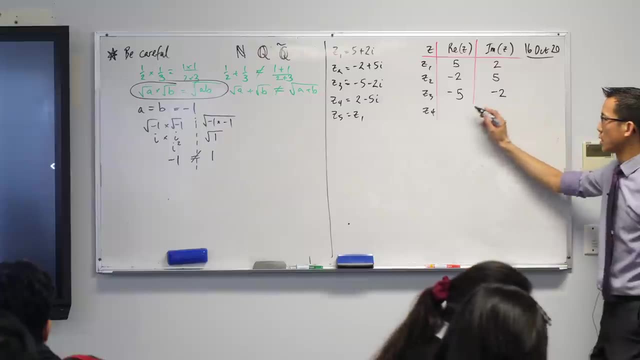 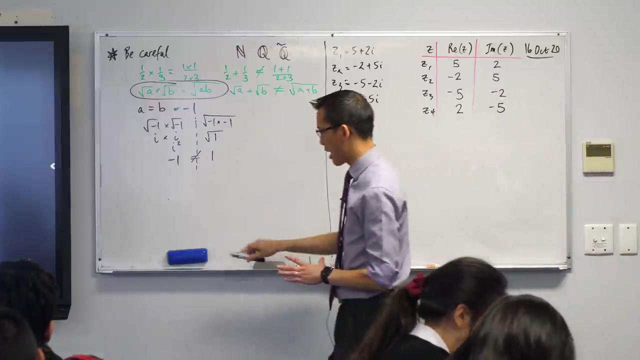 Negative 2 and positive 5.. Yeah, Next one down: Negative 5, negative 2.. Last one here: 2 and negative 5.. You okay with that? I want you to stare really hard. I'm inviting you to kind of be like. 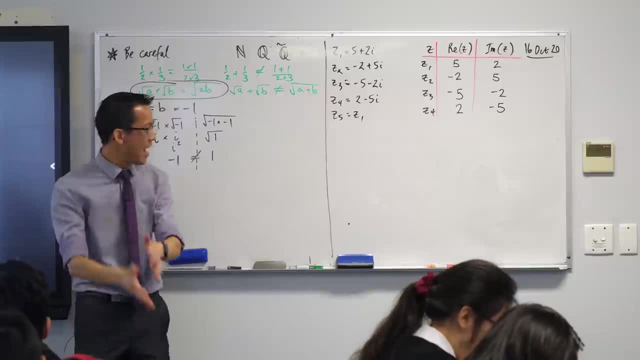 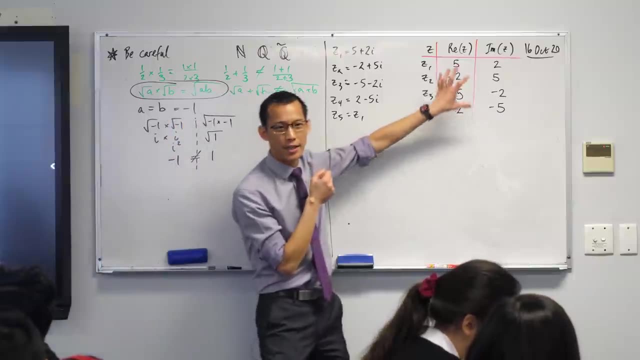 Brown, like that botanist who was staring down his microscope and he was like: What's going on here? Is there something more than what I can see? Is there something invisible underneath this that's driving this process? These are not just random numbers, right? What do you notice? What do you wonder when you have a look at these? 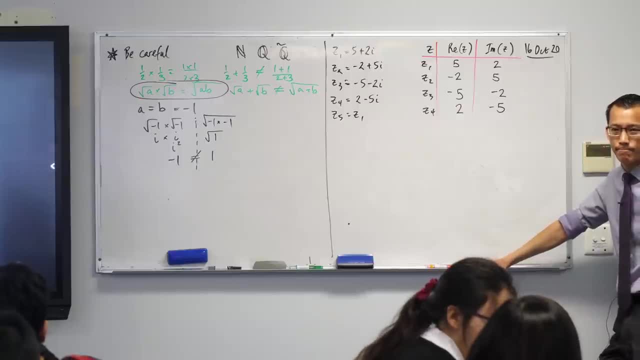 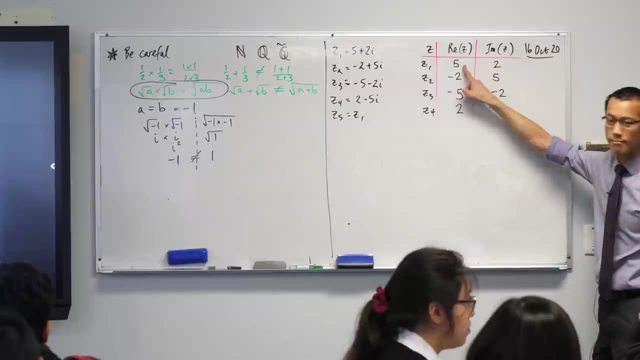 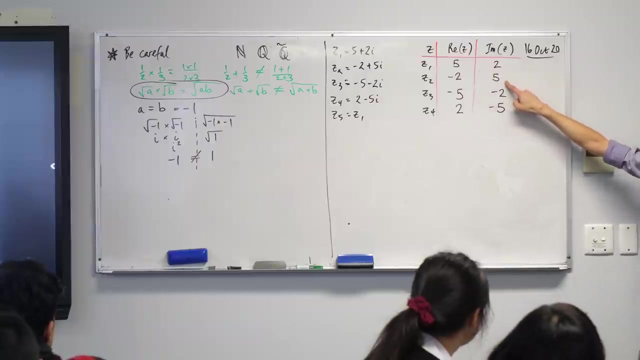 Does anyone notice any patterns? What do you see? What do you think? Start us off? Huh, okay, so real part of this, one imaginary part of this one Real part, imaginary part, real part, imaginary part, and you could extend it all the way around, right? 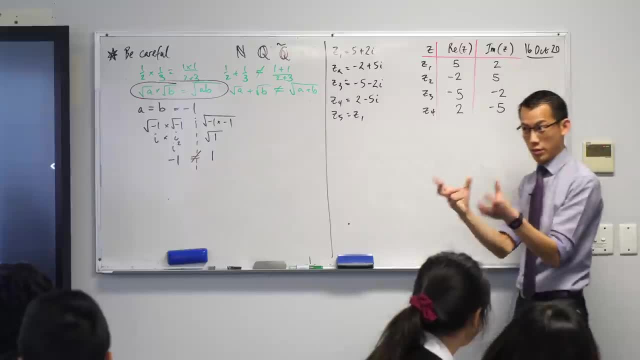 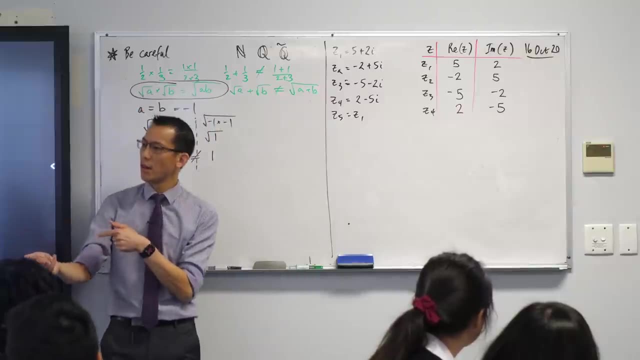 Here comes the real part and then the imaginary part. Good, So we're noticing, there's this relationship. Is there anything else that you notice? Every two cycles, it multiplies by minus 4.. Every two cycles, it multiplies by minus 4.. 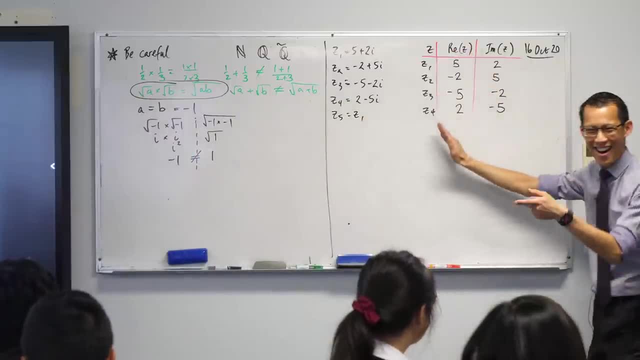 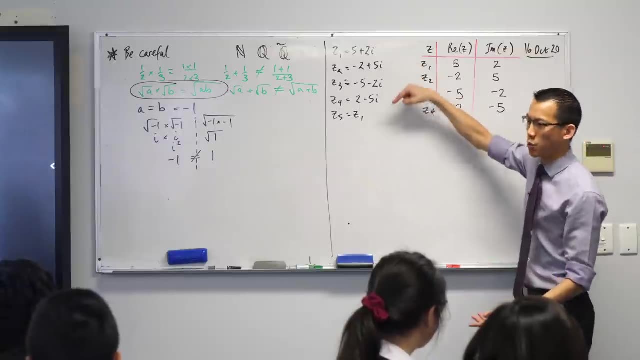 Every two cycles. let me say that again: Angad Every two cycles of multiplying by i, you're essentially multiplying by minus 1.. That makes sense, because each time we progress we're multiplying by i. So if you do it twice, you're multiplying by i, squared. 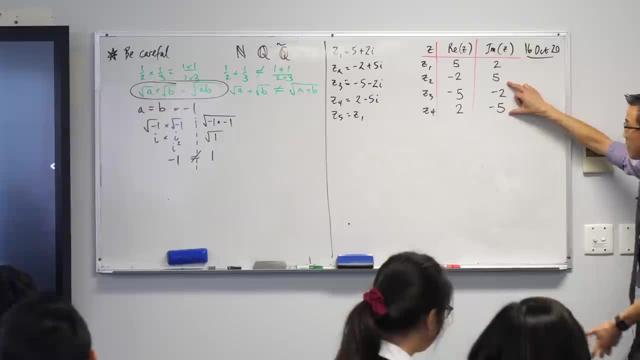 So if you have a look at these two, yeah, you see the flipping of signs. If you look at these two flipping of signs and you can do it with any like as long as your gap is 2, right. 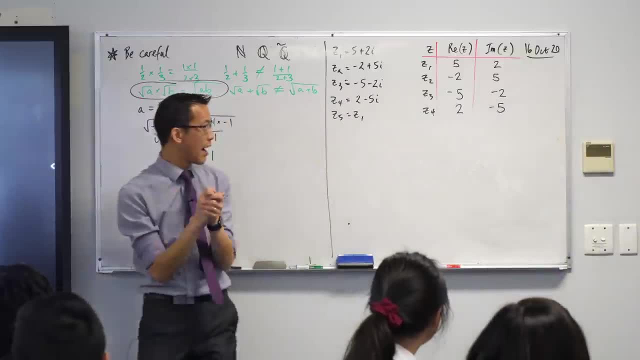 Hmm, Now, the last thing I want you to notice is I call these numbers something specific, right? I call them z1, z2.. There's the first number, the second number, the third and the third, And then the fourth. 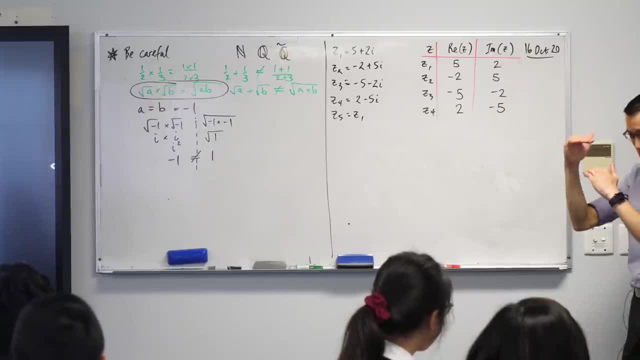 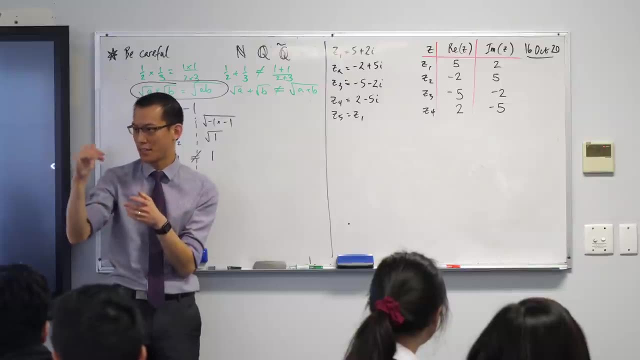 flipping of signs, and you can do it with any like so long as your gap is 2, right? Hmm, Now, the last thing I want you to notice is I call these numbers something specific, right? I call them z1, z2.. There's the first number, the second number, the third and then the fourth. 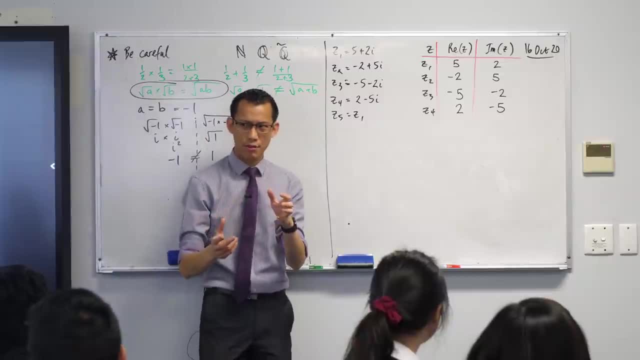 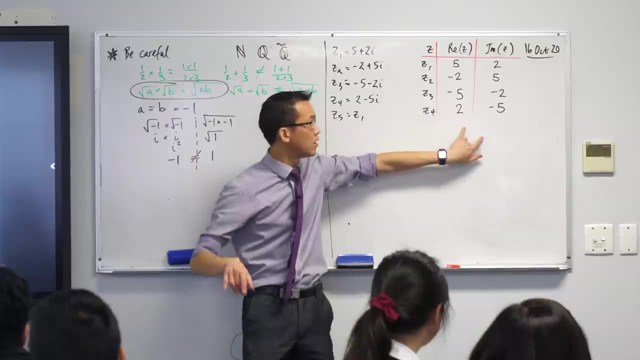 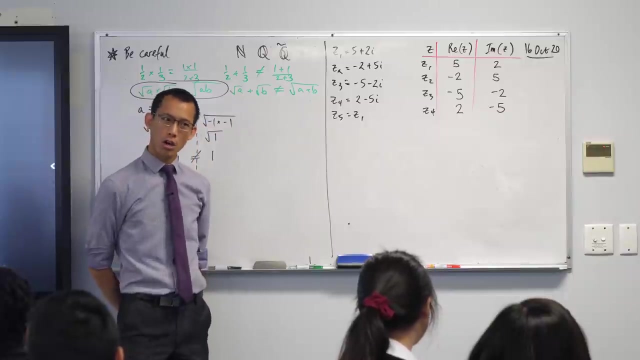 If you were to imagine, because they aren't, but if they were, if you were to imagine these guys as coordinates, like it's a pair of numbers, each time coordinates on like a Cartesian plane, where would these numbers go And what relationship would there be between them? 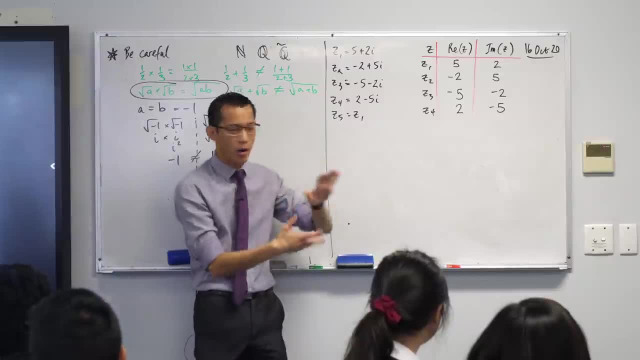 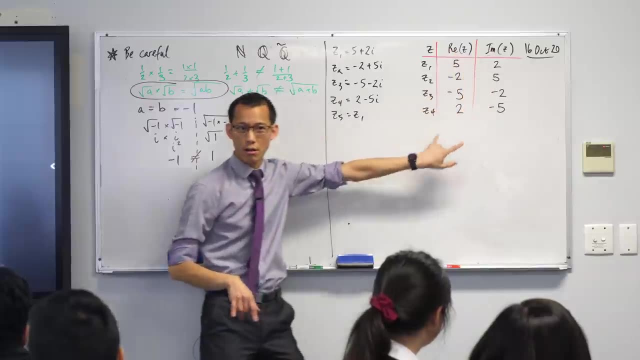 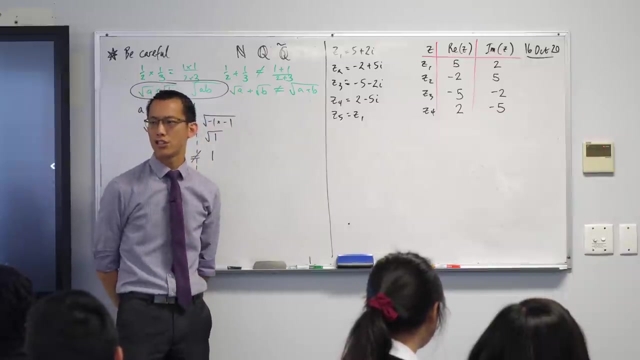 If you were to imagine, because they aren't, but if they were, if you were to imagine these guys as coordinates, like it's a pair of numbers, each time coordinates on like a Cartesian plane, where would these numbers go And what relationship would there be between them? 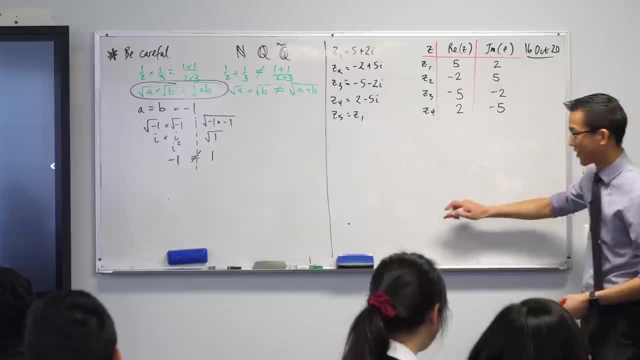 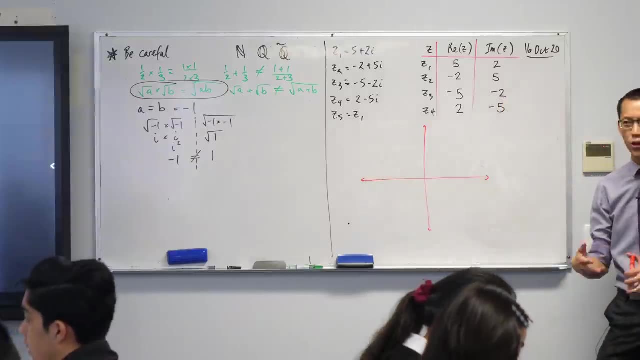 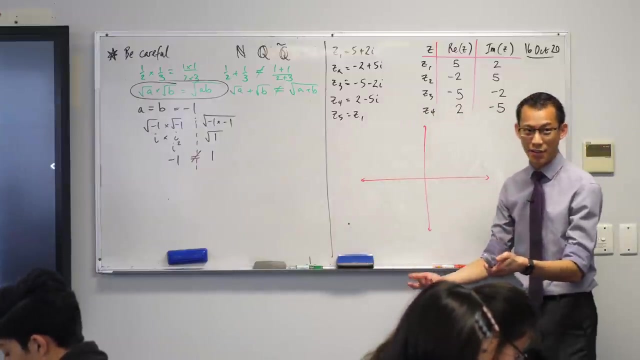 Hear me, Draw me a Cartesian plane just underneath where you got this right And, for the sake of the conclusion we're about to draw right, Get some decent scale on this. If you have a grid book, then you're at an advantage, but I don't. 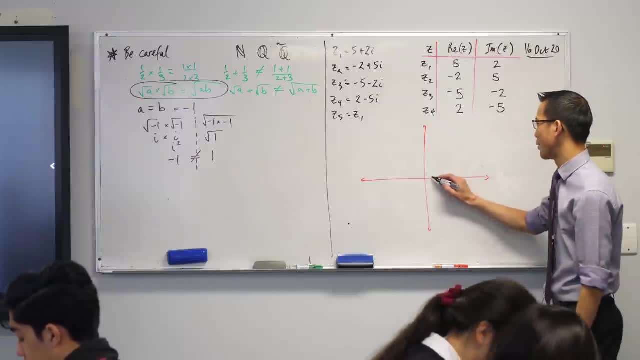 And in the HSC you won't. So I'm going to draw some quick little indicators for me of scale here And because of the numbers we've got, you're going to have to go up to 5 everywhere. so go ahead. 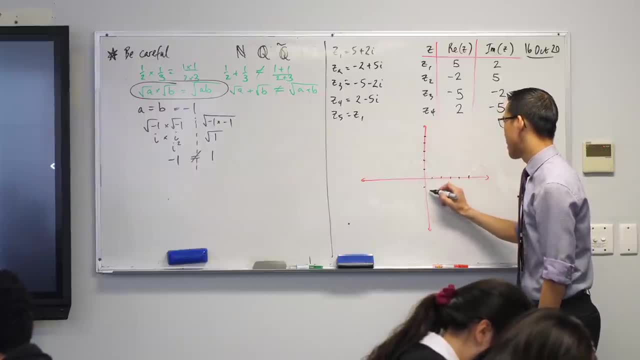 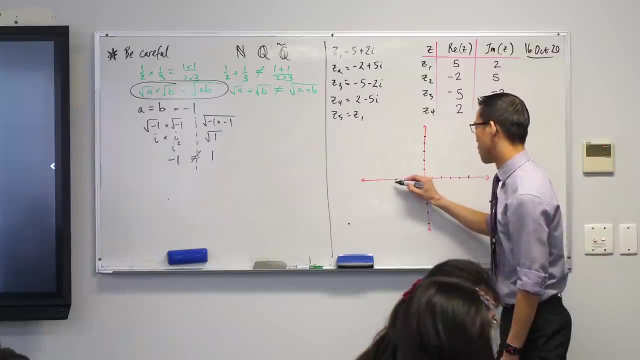 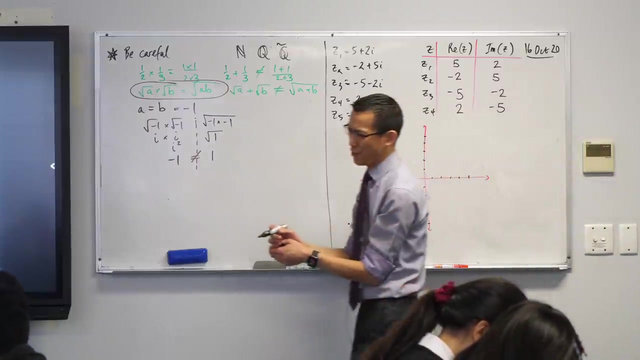 and put that, so you've got something consistent, and a ruler would be enormously helpful for this Right. I mean, one of the cheating things is it's actually a lot easier to draw accurate diagrams on a whiteboard because they're huge When you're doing it small. you really should. 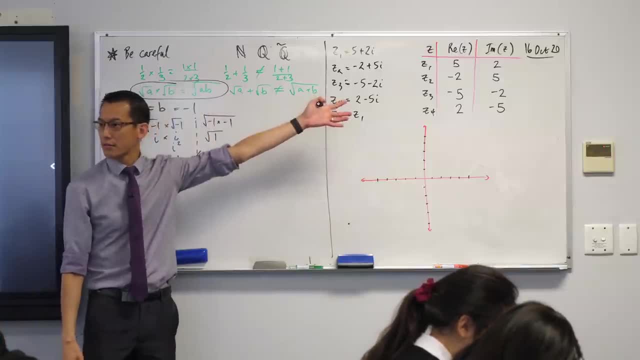 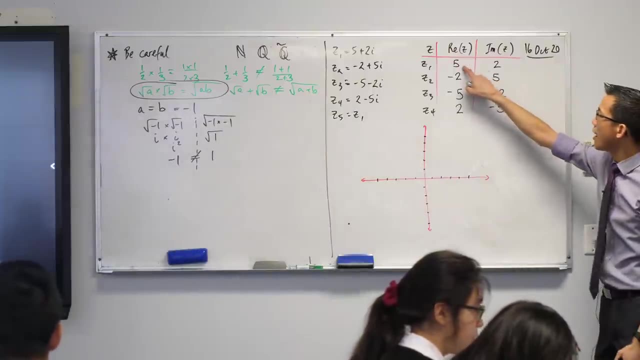 If you want a straight line, use a ruler So you can see. I've got values on my scale up to 5 in all directions. So where would this number here? 5,2, where would that be The first number? it's going to be 5,2.. 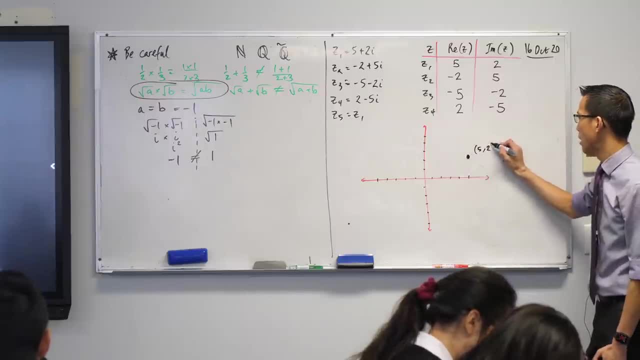 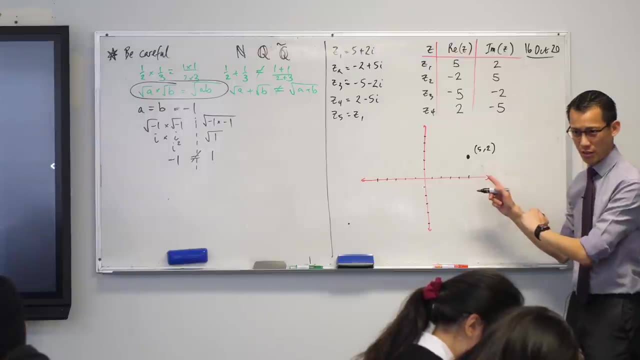 It's going to be there, Is that okay? Call that 5,2.. The first number over here. where's the second number, Negative 2,5.. That's going to be. point to it. where's it going to be? 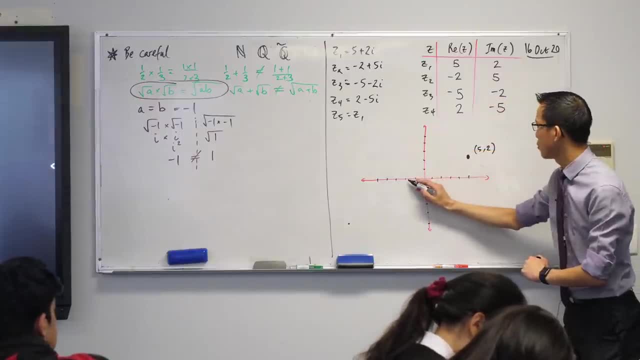 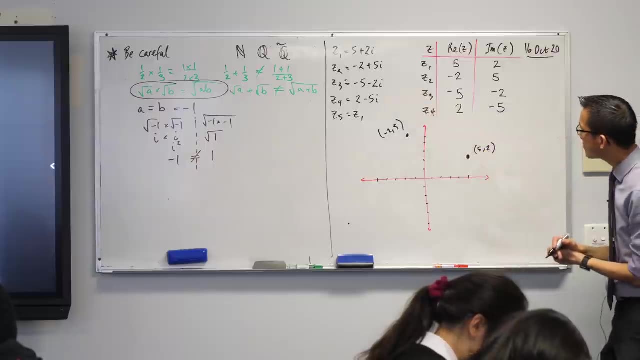 It's going to be up here, right? So I'm going to go negative 2,5.. So about there-ish Negative 2,5. And then I'm just going to keep going around. This first number's over here. 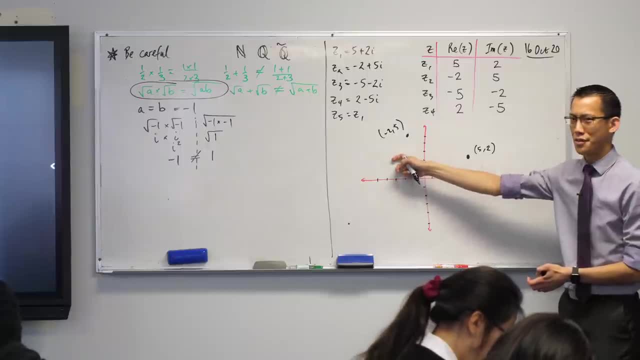 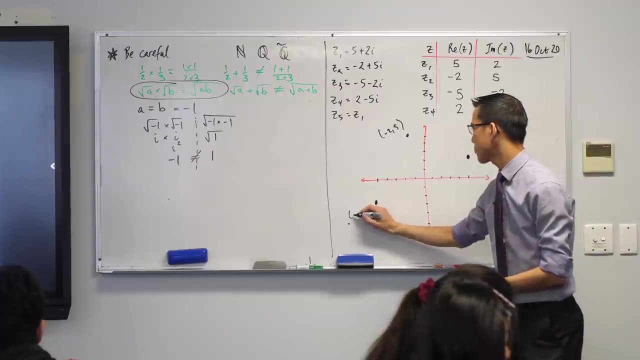 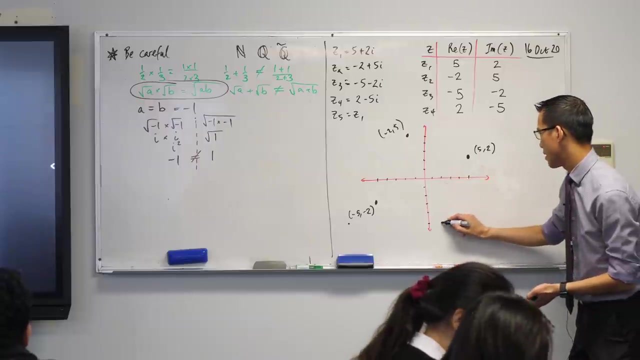 Second number's over here. Third number is Down here, isn't it? Negative 5, negative 2.. Some over here: Negative 5, negative 2.. And then finally, 2, negative 5 will be here. 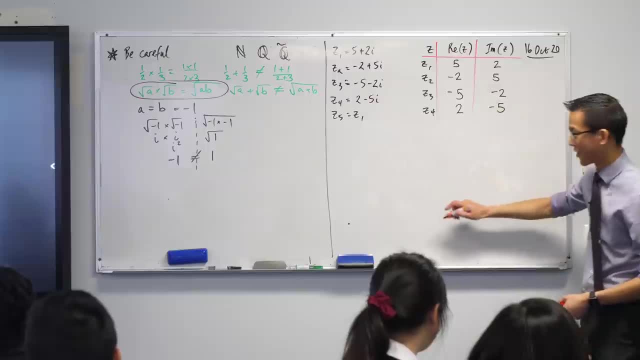 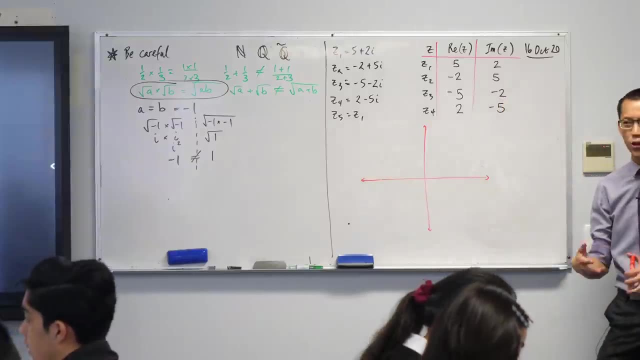 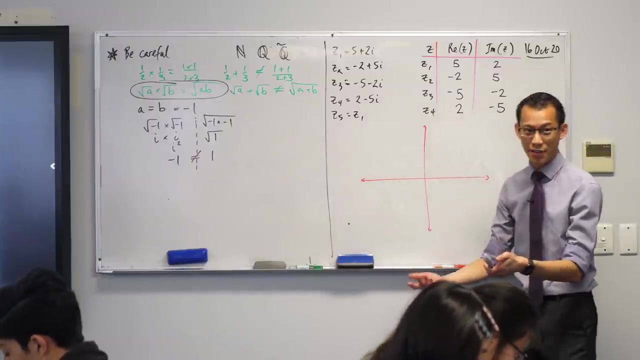 Cue me. Draw me a Cartesian plane just underneath where you got this right And, for the sake of the conclusion we're about to draw right, Get some decent scale on this. If you have a grid book, then you're at an advantage, but I don't. 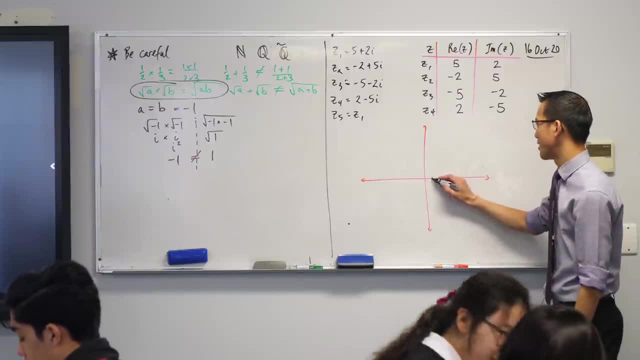 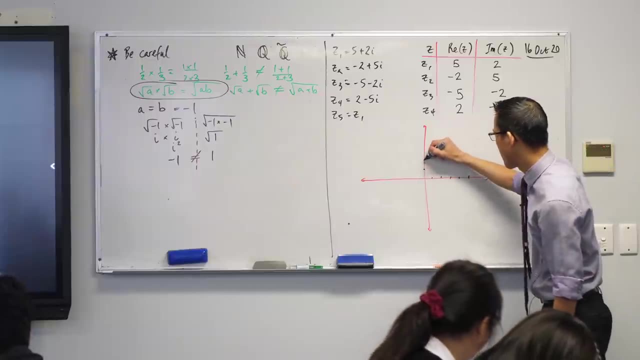 And in the HSC you won't. So I'm going to draw some quick little indicators for me of scale here and because of the numbers we've got, you're gonna have to go up to five everywhere. So go ahead and put that, so you've got something consistent and a 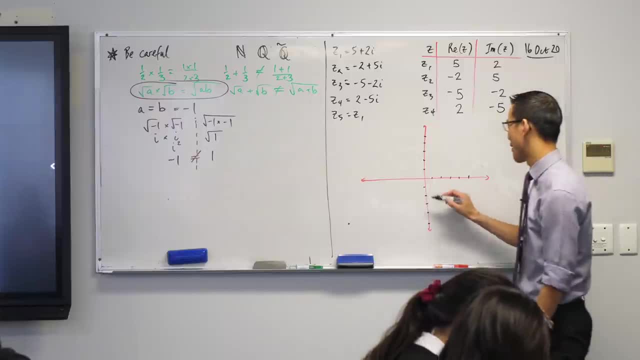 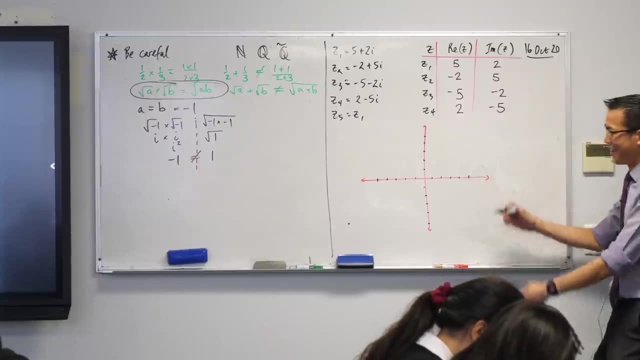 ruler would be enormously helpful for this Right. I mean, one of the cheating things is it's actually a lot easier to draw accurate diagrams on a whiteboard because they're huge When you're doing it small. you really should. If you want a straight line, use a ruler. 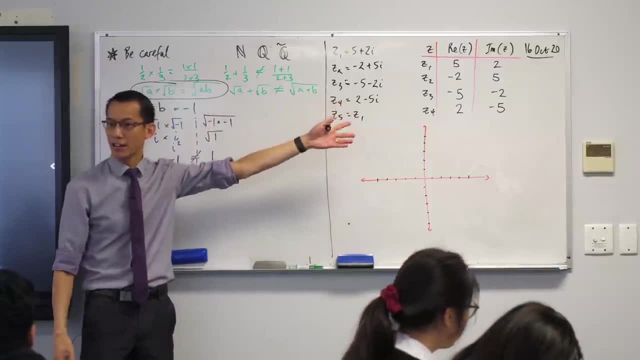 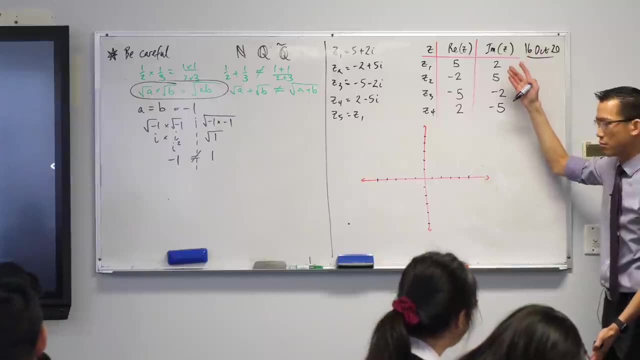 So you can see I've got, you know, values on my scale up to five in all directions. So where would this number here? five comma two, where would that be The first number? It's gonna be, I mean five comma two. It's gonna be there, Is that okay? 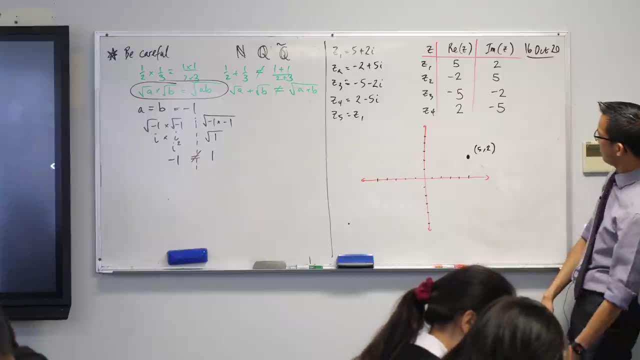 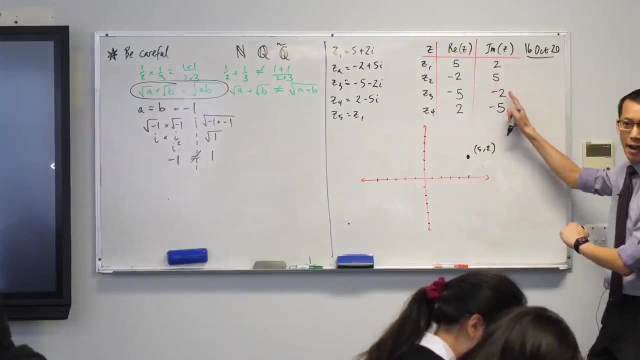 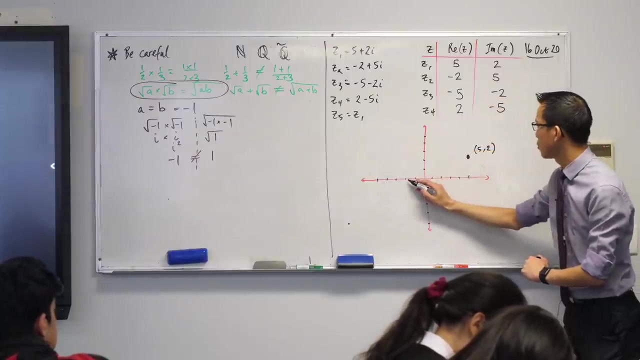 Call that five comma two. First number over here. Where's the second number? Negative two, five. That's gonna be. point to it. where's it gonna be? It's gonna be, it's gonna be up here, right, So I'm gonna go negative. two comma five. 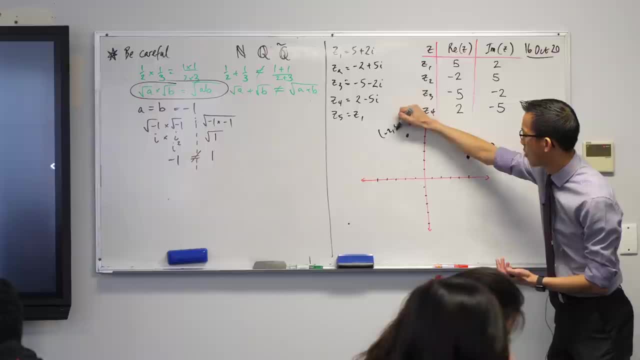 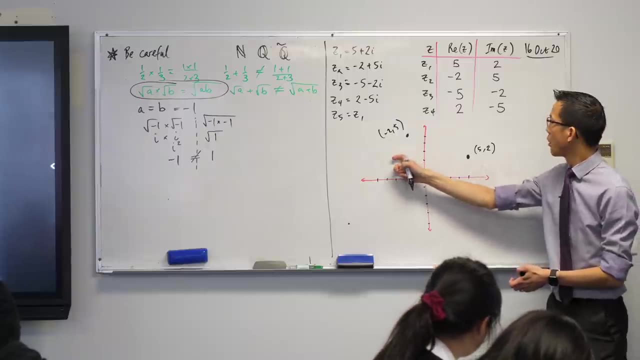 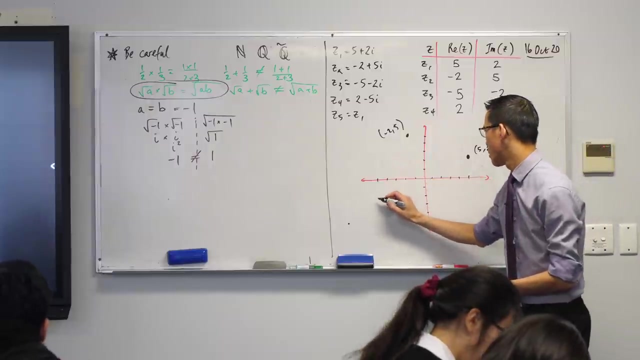 So about there-ish: Negative two, comma five, right, And then I'm just gonna keep going around, right, This first number's over here. second number's over here, third number- Third number is down here, isn't it? Negative five, negative two. So I'm over here. 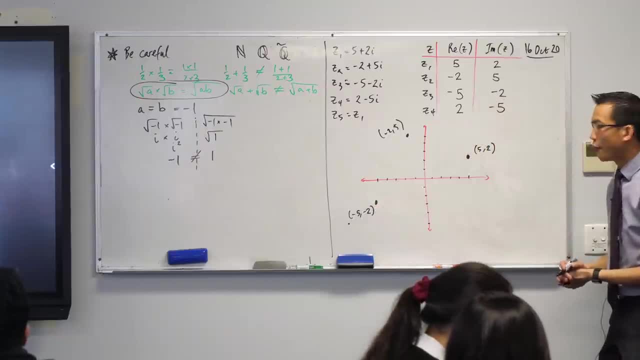 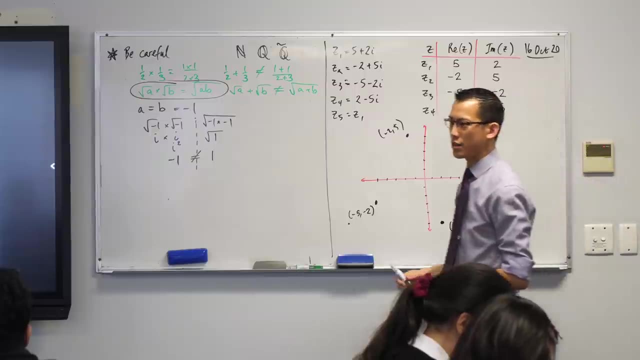 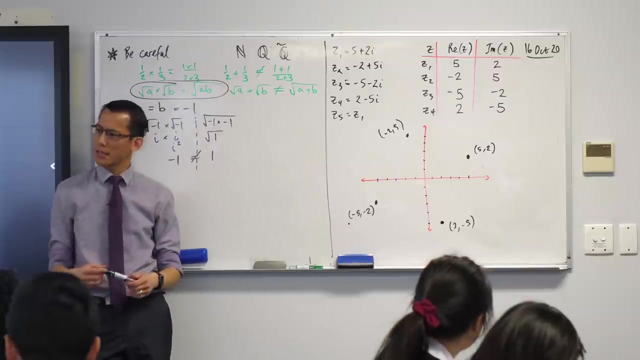 Negative five, negative two And then finally two comma negative five will be here. Isn't that strange that the first number it's in the first quadrant. I just defined that for you. But if the first number's in the first quadrant, then the second number ends up in the second quadrant. 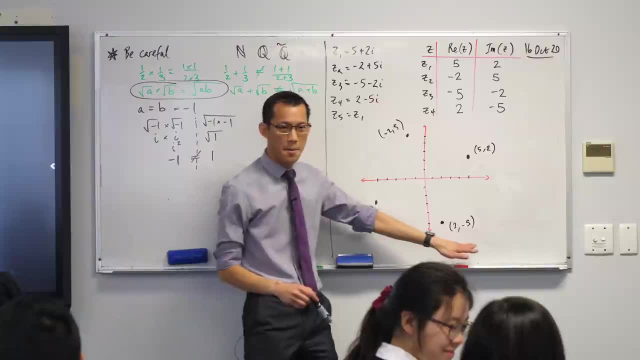 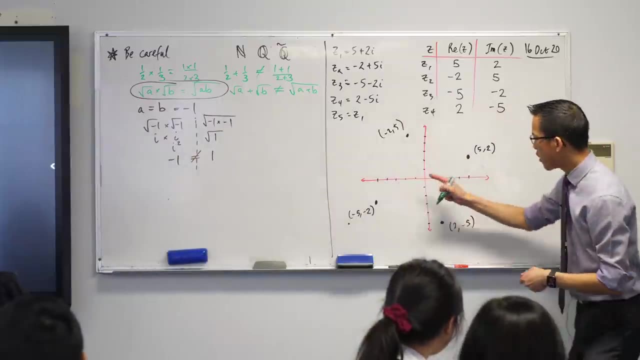 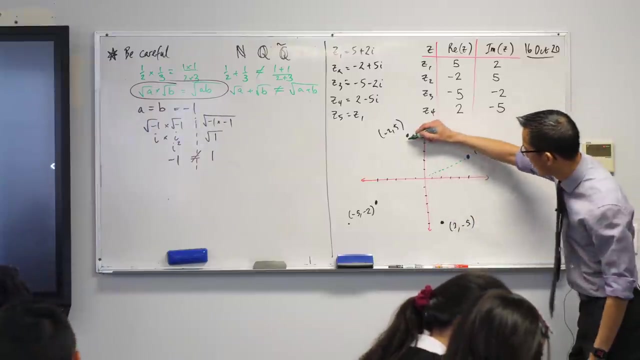 And the third number's in the third quadrant And the fourth number's in the fourth quadrant. Put one more thing onto your diagram just to help me out, right From the origin here. if you imagine a line extending upwards right to my point over here And then another line or an interval, I should say that goes from the origin to my next point. 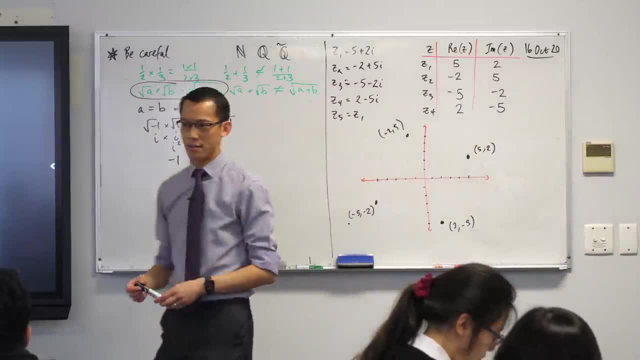 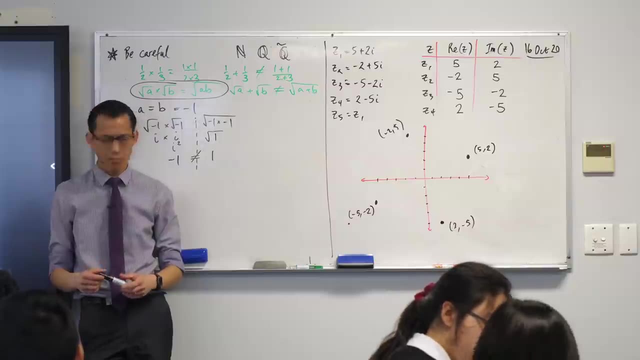 Isn't that strange that the first number it's in the first quadrant? I just defined that for you. But if the first number's in the first quadrant, then the second number ends up in the second quadrant And the third number's in the third quadrant. 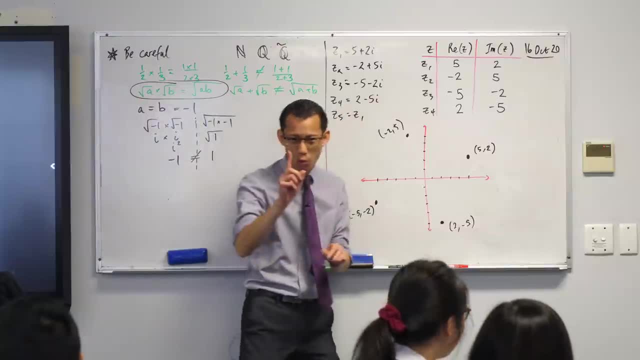 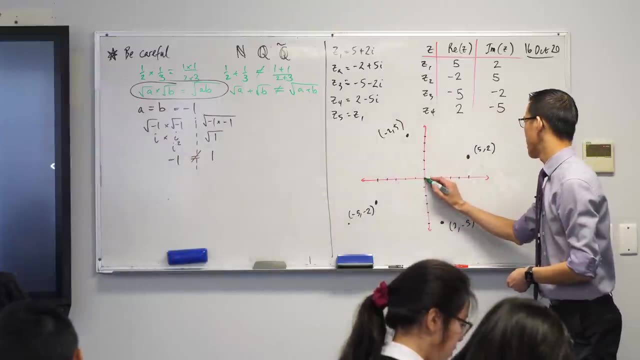 And the fourth number And the fourth number's in the fourth quadrant. Put one more thing onto your diagram just to help me out right From the origin here. if you imagine a line extending upwards right To my point over here, 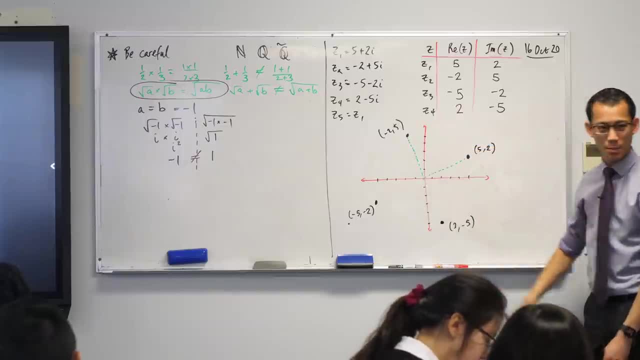 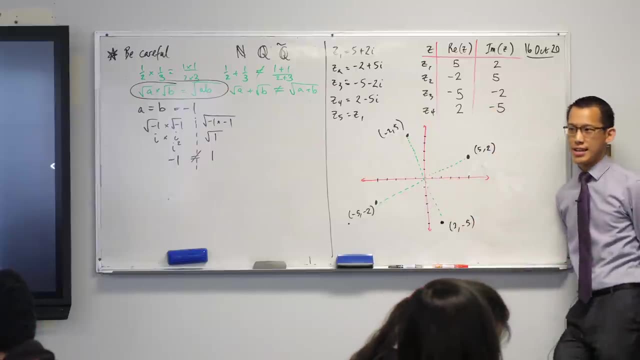 And then another line or an interval. I should say that goes from the origin to my next point. And then another line over here, another interval, another interval, right, Can you see And remember the z5, the z5 I asked you to calculate. 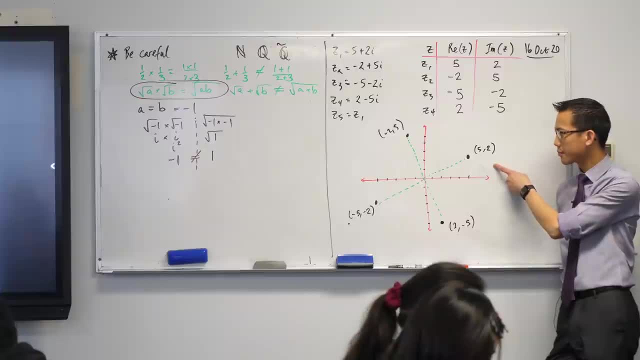 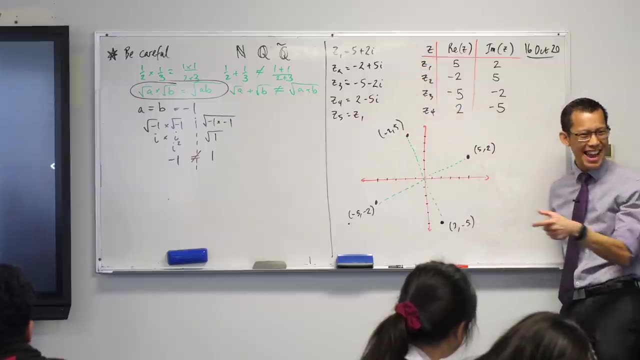 it ends up back over here, right, It ends up at 5,2.. What is the operation that takes you through these numbers? The answer is: I'm multiplying by i. But now, if you think of this not as an arithmetic problem, 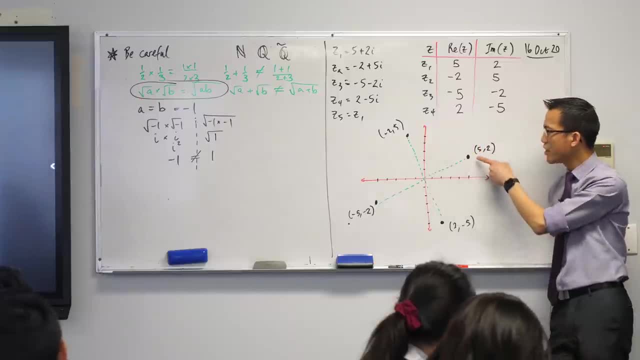 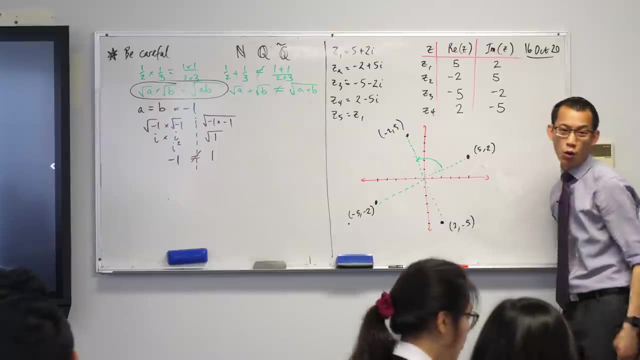 but as a geometric problem, what operation gets you from the first number to the second? It's rotating 90 degrees. I'm rotating 90 degrees, or pi on 2 radians right. And then what? I'm going anticlockwise as well. 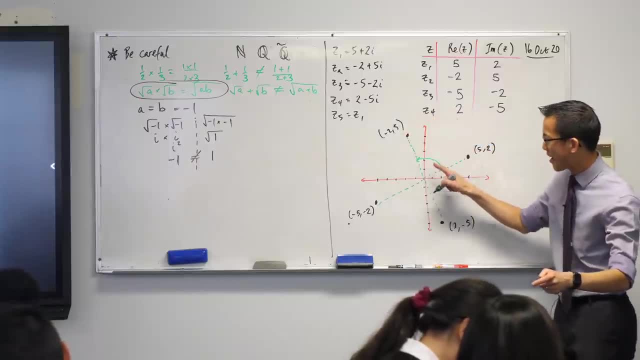 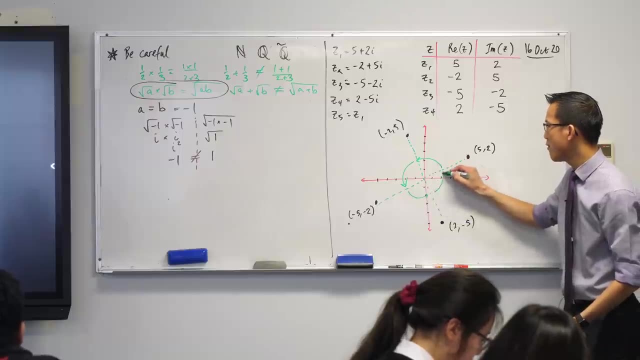 because I started here and I ended up in the second quadrant, And then I do it again because I'm still multiplying by i, I rotate again, and then I rotate again. If you ever wondered why, when we do compass bearings right. 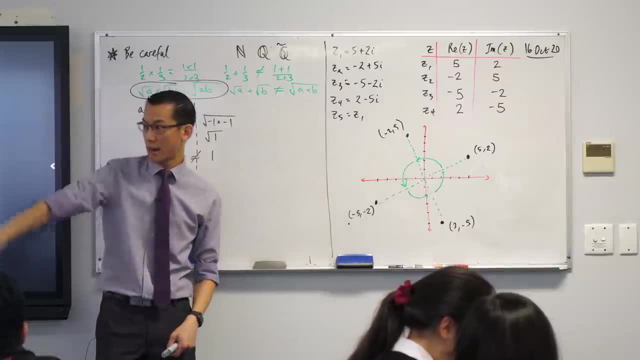 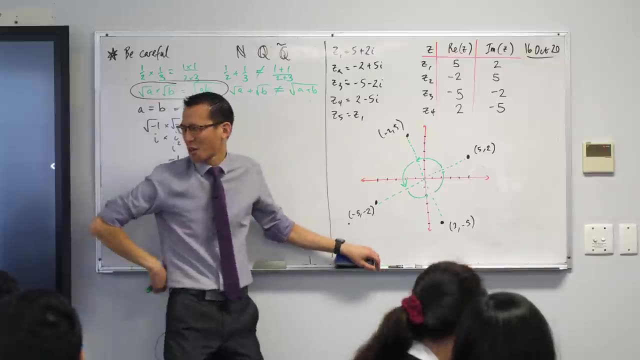 We say: start from true north and then go clockwise, right. But then for some reason, when we moved into the Cartesian plane, we then said: actually we want you to go anticlockwise, Don't worry about why. We just want to mess with you and make things as hard and arbitrary as possible. 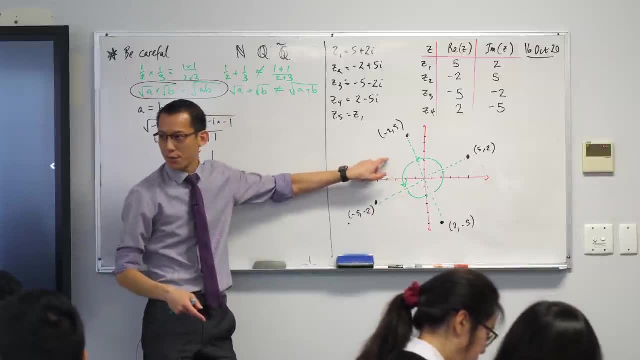 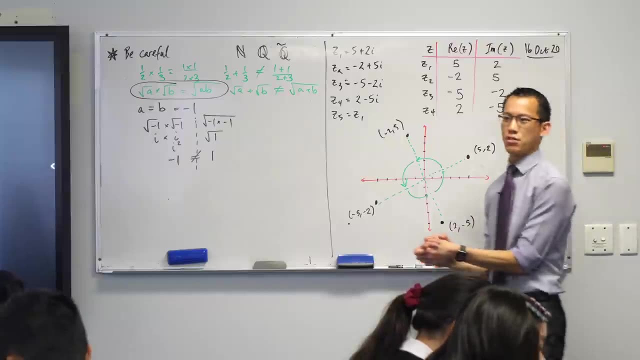 Why are we going the opposite direction? The answer is because of this multiplication by i. it's rotating you around. Do you remember when we had a look at those water molecules? right, The problem, the reason why they were invisible, is because they were too small. 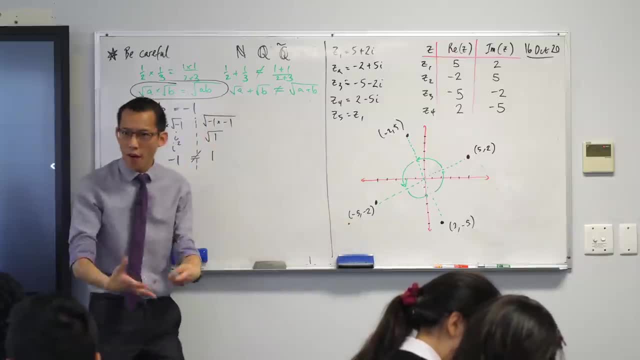 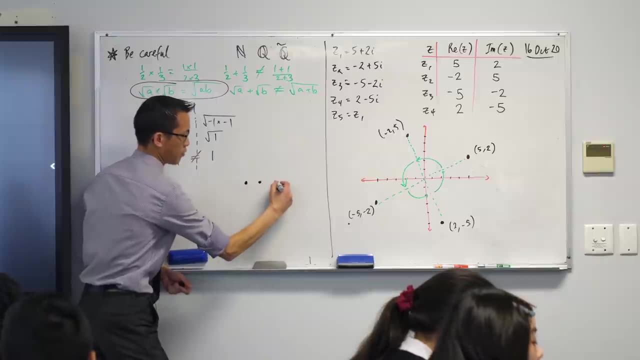 Do you remember that They were too small? Why could we never find? why were these complex numbers invisible to us? Well, if you want to think about the natural numbers 1,, 2,, 3,, 4,, 5, and so on, right, 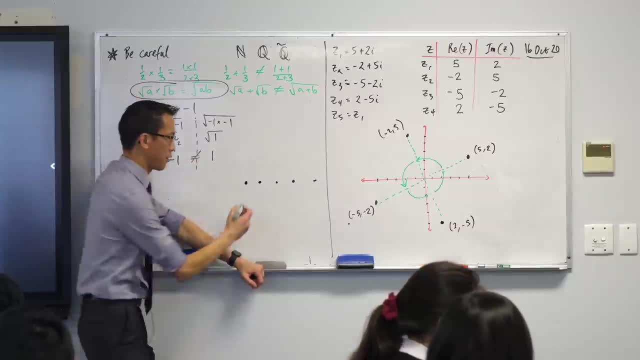 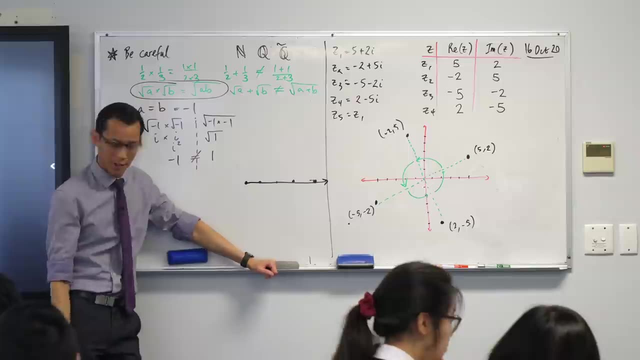 You can imagine sort of progressing along. Then we add the rational numbers. you sort of fill in the gap Right. All of those numbers are filled in between them. Then when we said we add the integers, we could say you can go off. you know, if that's 0 you can go off in the other direction as well. 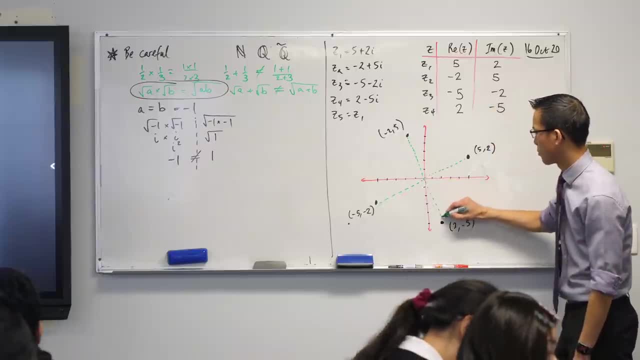 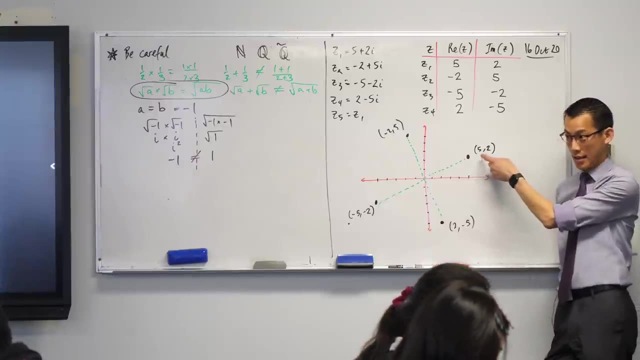 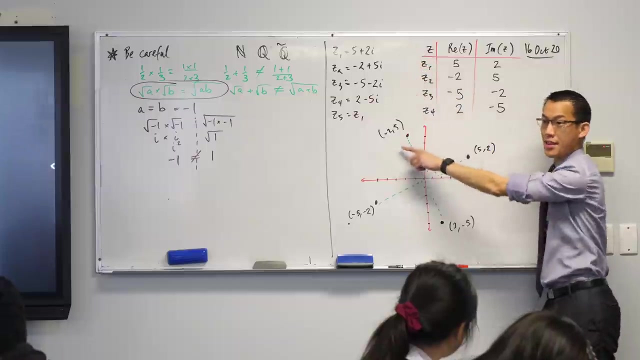 And then another line over here, another interval, another interval, right, Can you see and remember the z five, the z five I asked you to calculate. it ends up back over here, Right, Ends up at five comma two. What is the operation that takes you from through these numbers? 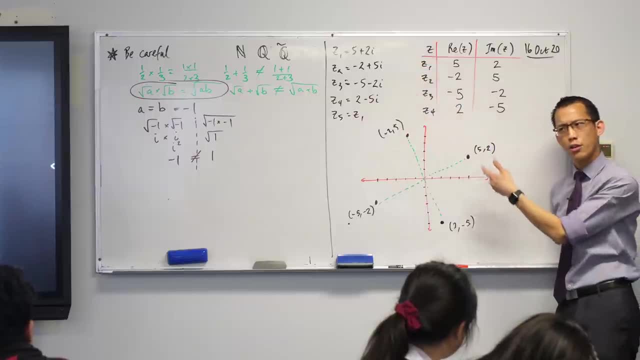 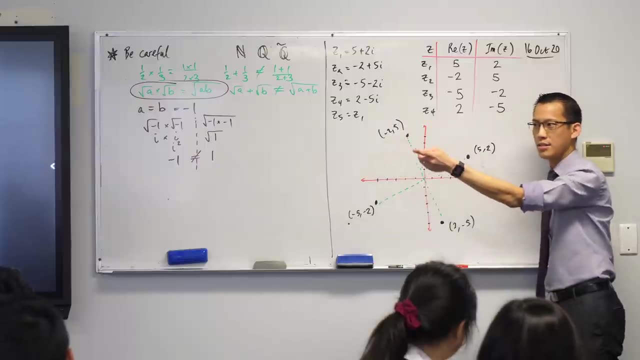 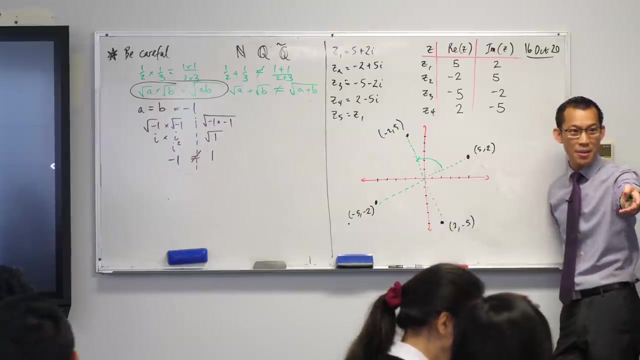 The answer is: I'm multiplying by i. but now, if you think of this not as an arithmetic problem, but as a geometric problem, what operation gets you from the first number to the second? It's: I'm rotating 90 degrees, or pi, on two radians right. And then what? Yeah, 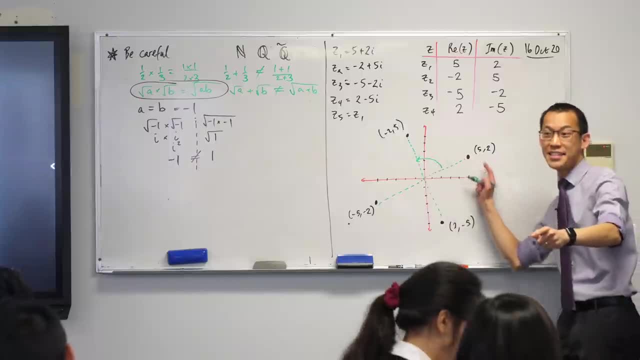 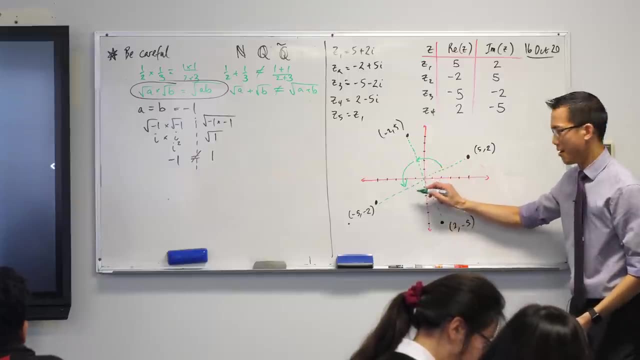 I'm going anti-clockwise as well, because I started here and I ended up in the second quadrant, And then I do it again, because I'm still multiplying by i, I rotate again, and then I rotate again. If you ever wondered why. 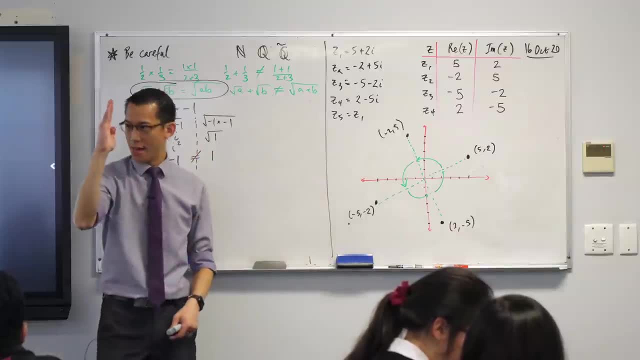 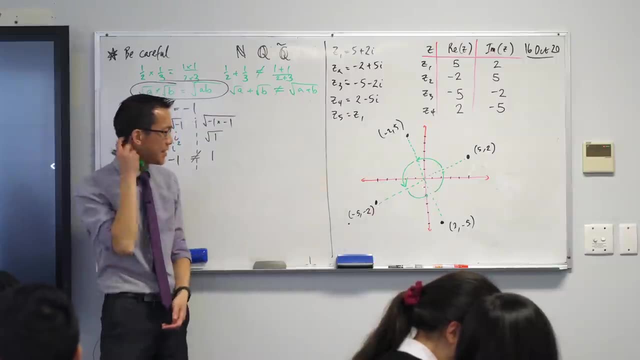 when we do compass bearings right, we say start from true north and then go clockwise, right. But then for some reason, when we moved into the Cartesian plane, we then said: actually we want you to go anti-clockwise, Don't worry about why. just we just want to mess with you and make things as hard and arbitrary as possible. 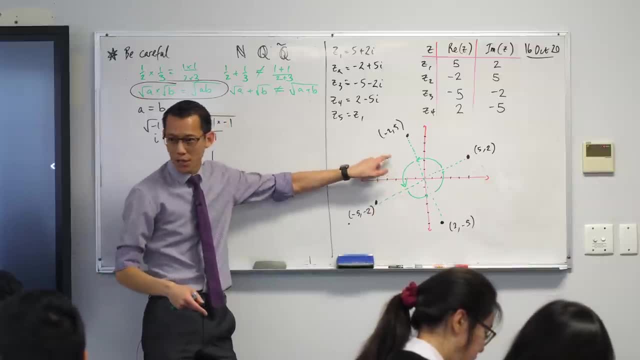 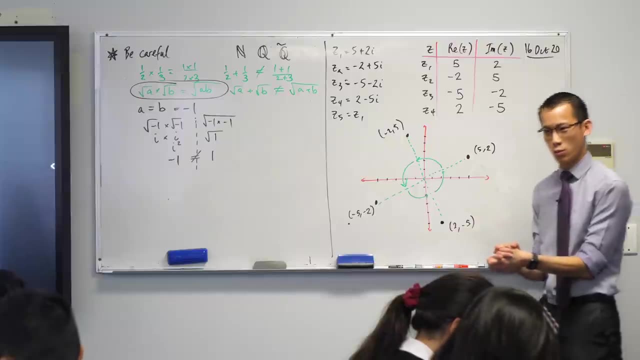 Why are we going the opposite direction? The answer is because of this multiplication by i. it's rotating you around. Do you remember when we had a look at those water molecules? right, The problem, the reason why they're invisible, is because they were too small. Do you remember that They were too small? 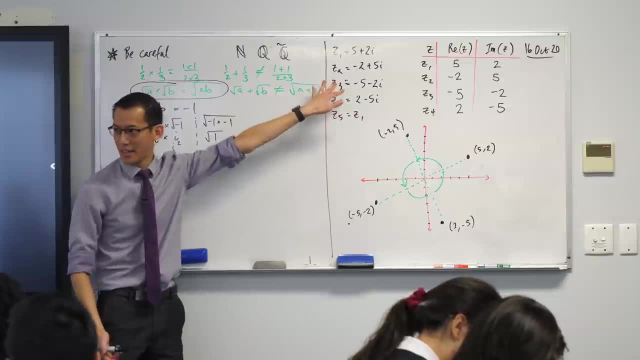 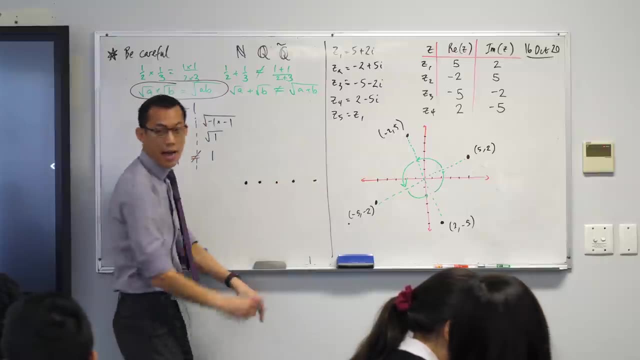 Why could we never find? why were these complex numbers invisible to us? Well, if you want to think about the natural numbers one, two, three, four, five and so on, right, You can imagine sort of progressing along. 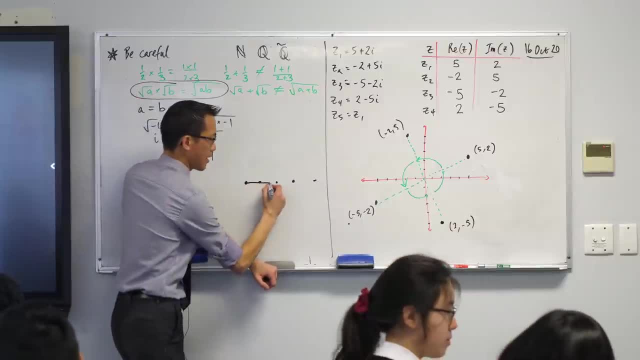 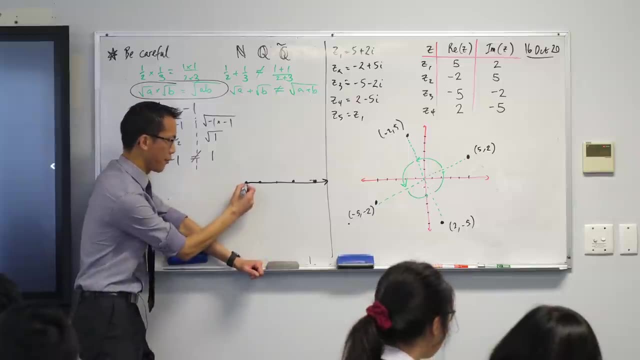 Then we add the rational numbers, numbers you sort of fill in the gaps, right, all of those numbers are filled in between them. then, when we said we add the integers, we can say you can go off. you know, if that's zero, you can go off in the the other direction as well. and 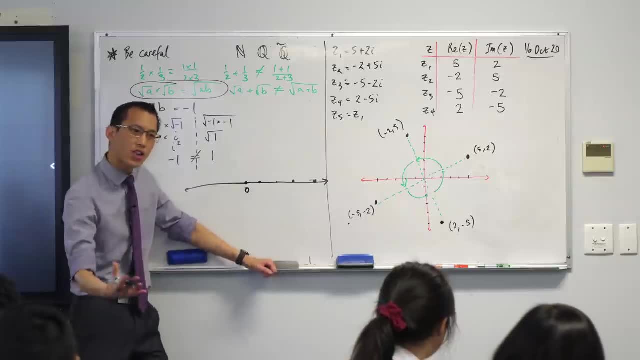 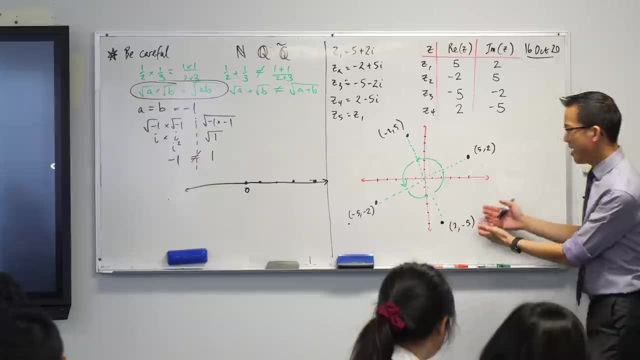 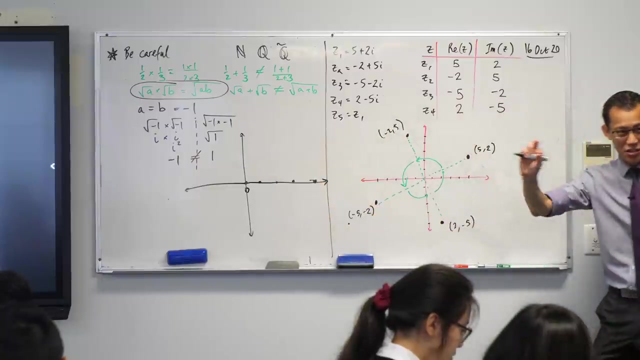 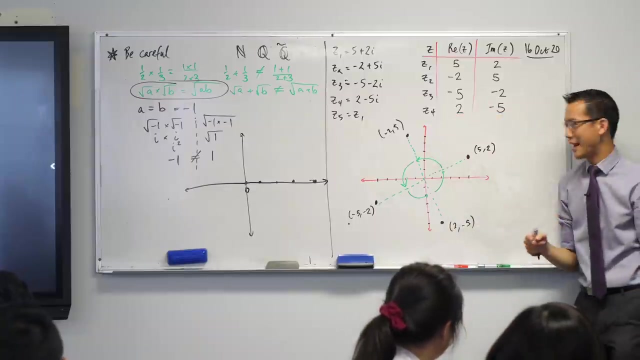 this is what we call the number line, right, but these complex numbers that we are searching for, they're not anywhere on this number line. they're actually on a number plane. numbers are not one-dimensional, they can actually exist in two dimensions. what you've drawn here you might have noticed. I very